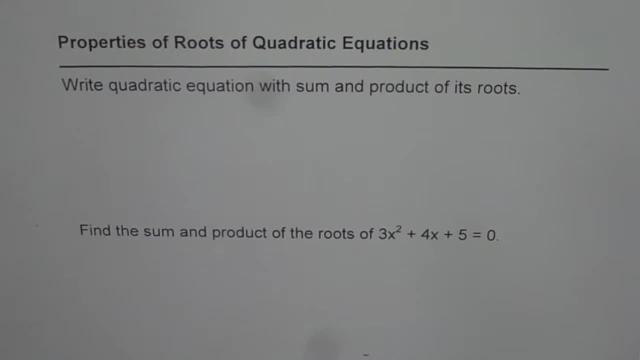 I am Anil Kumar and in this video we will try to understand properties of the roots of quadratic equations. We will also develop a relation between the two. The question here is: write quadratic equation with sum and product of its roots. Now let us assume that the roots of quadratic equations are x1 and x2.. 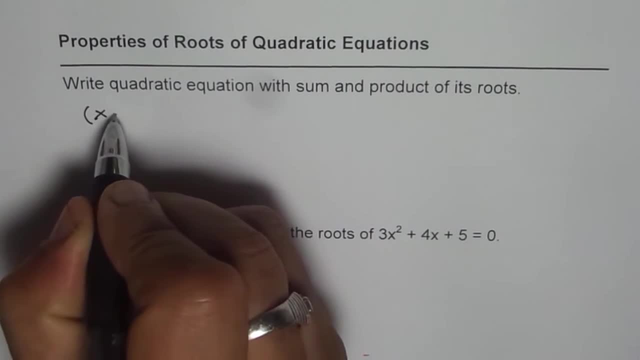 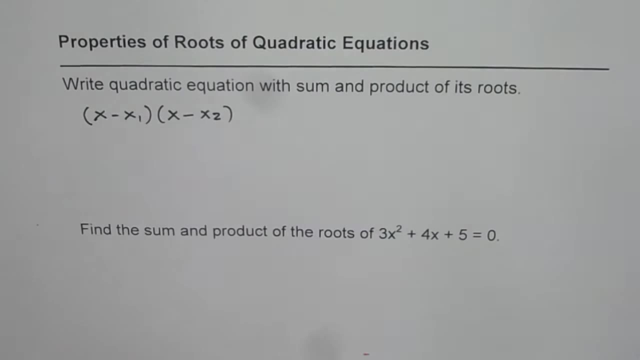 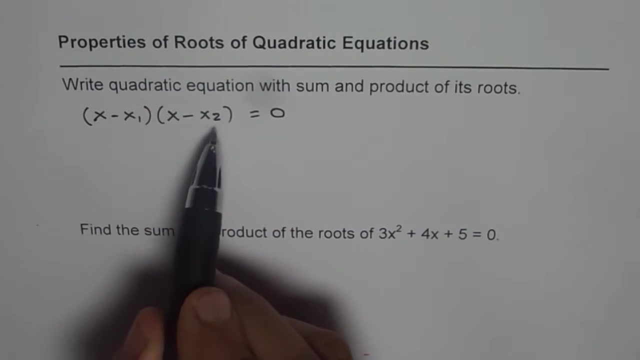 So if x1 and x2 are roots, then x minus x1 times x minus x2 will be factors, And when you multiply them you should get 0. So here x1 and x2 are roots. Since they are roots, x minus x1 times x minus x2 will be factors of that quadratic function. 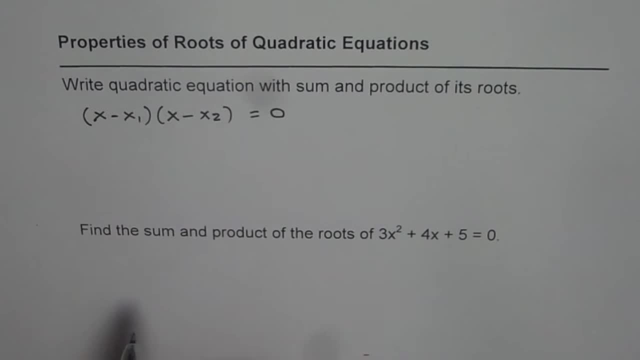 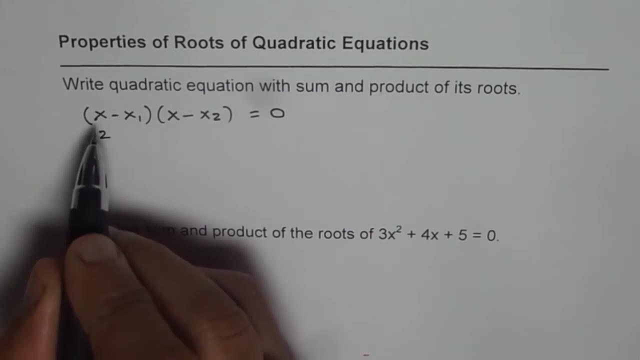 And when you multiply them you should get 0.. So let us assume that the roots of quadratic equations are x1 and x2.. So let us multiply and expand them. So x times x gives us x square, x times x2, the second root will be x2x. 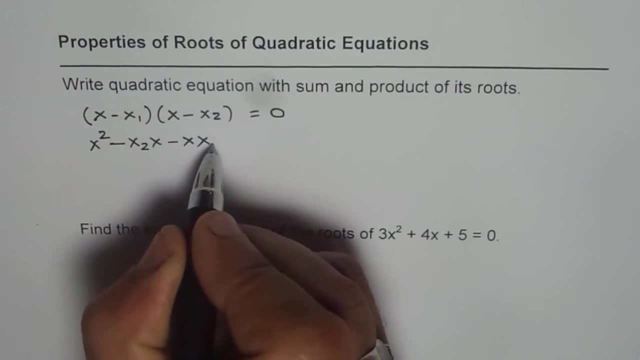 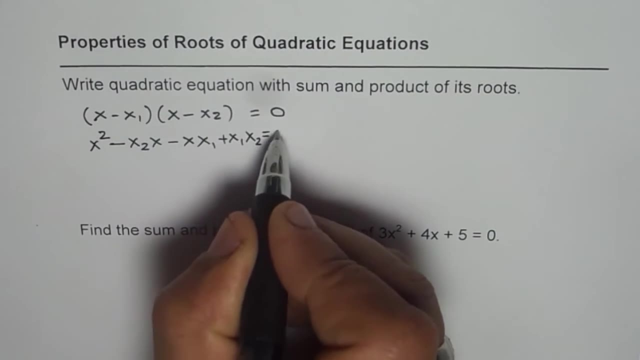 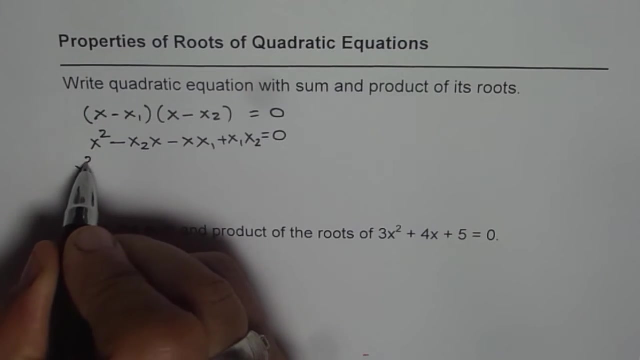 x1, x times x1 is xx1.. And when you multiply these two you get positive x1, x2 equals to 0.. Now if I factor x, then what do I get? I get x2.. Here, minus. 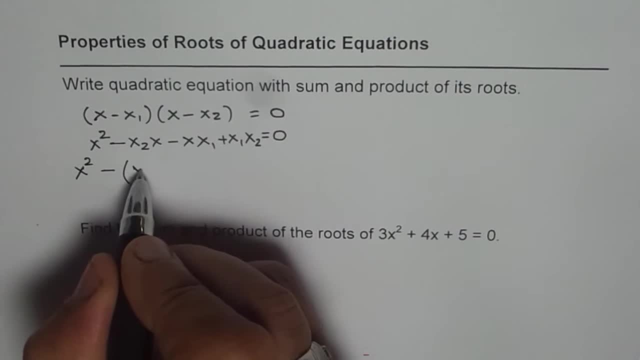 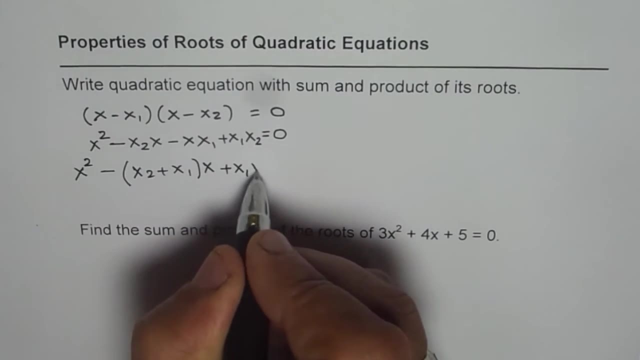 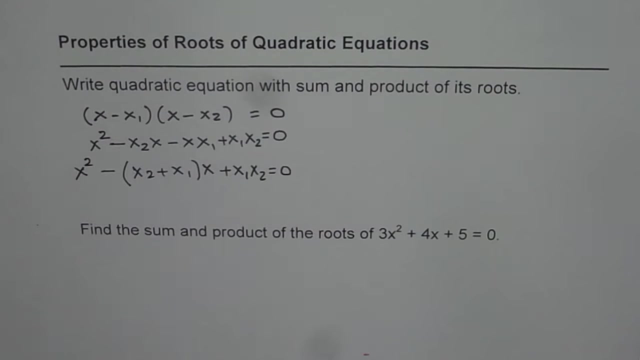 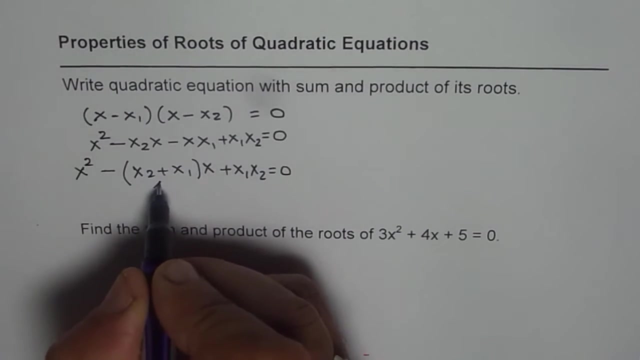 If I factor x, I get x2 plus x1. And here I have x1, x2 equals to 0.. Right Now, here you can see that we have written quadratic equation in the form of its roots. This is sum of roots. 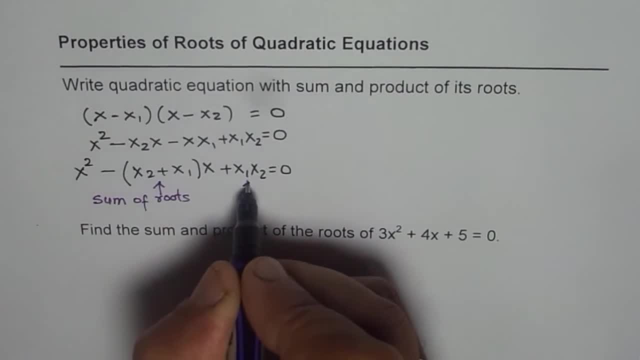 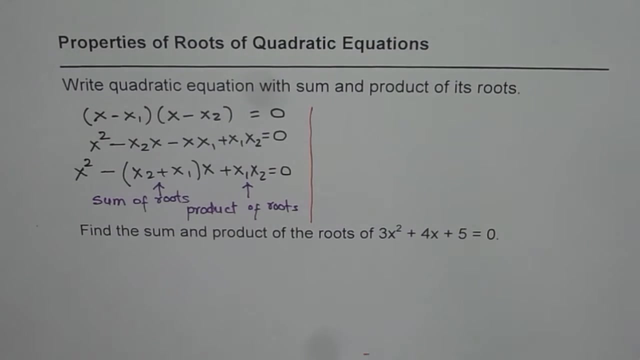 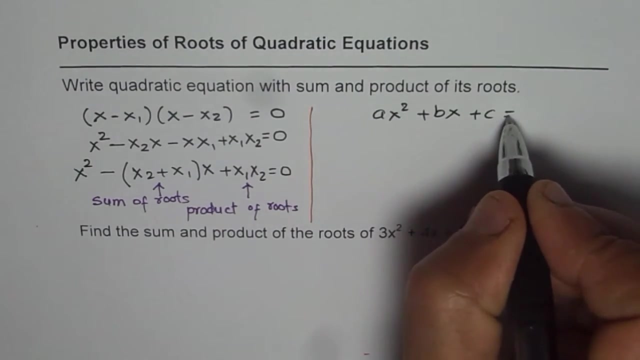 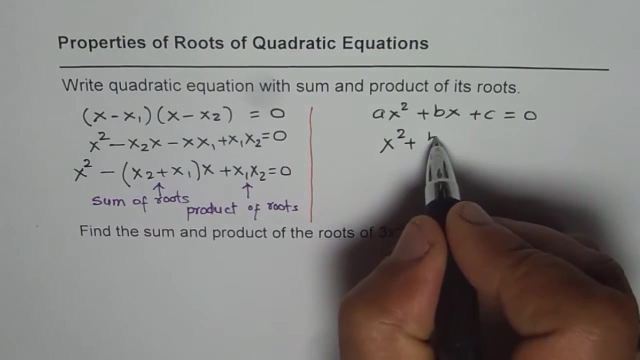 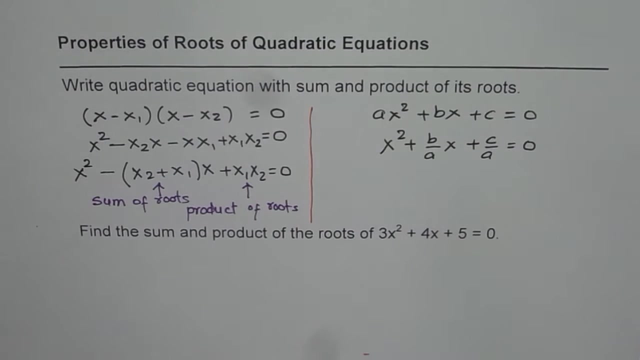 And how about this? That is product of roots, Correct. Now let us compare it with standard quadratic equation, which is: ax2 plus bx plus c equals to 0.. If I divide every term by a, I get x2.. So I get x2 plus b over ax, plus c over a equals to 0. 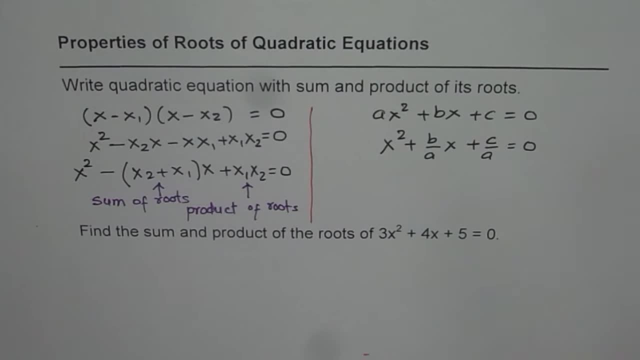 Now if I compare the two equations, then what is product equals to c over a And what is sum equals to Minus b over a. Right, So it is minus of sum is b over a. So comparing them, what do we get? 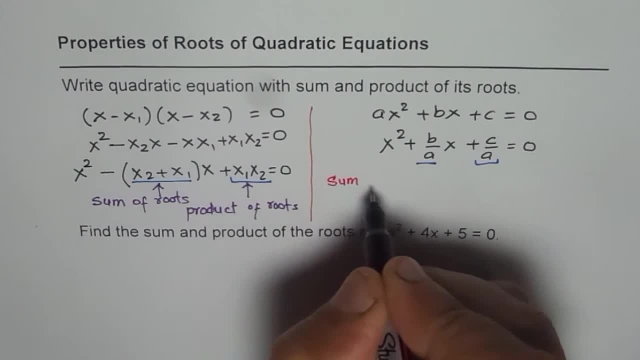 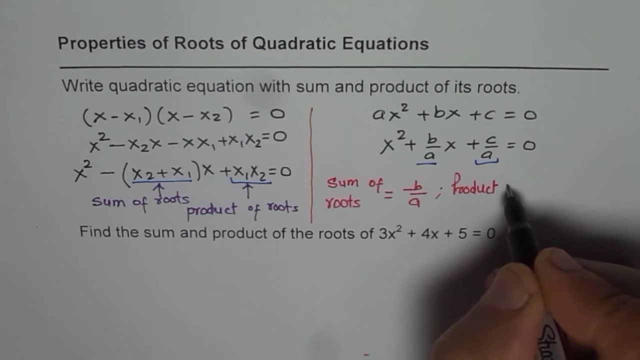 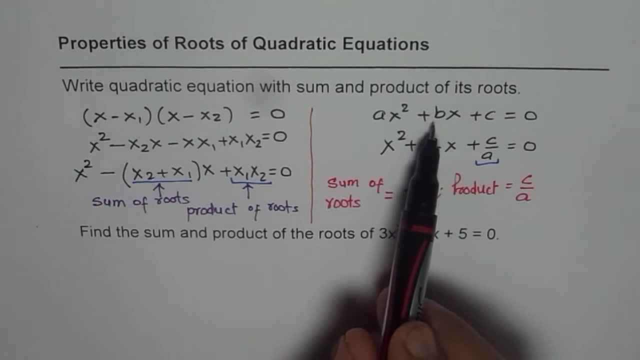 We get sum of roots equals to minus b over a And we get product as c over a. Do you see that? So we have linked the roots with the coefficients. in quadratic equation, a is the leading coefficient, b is the and c is the constant. 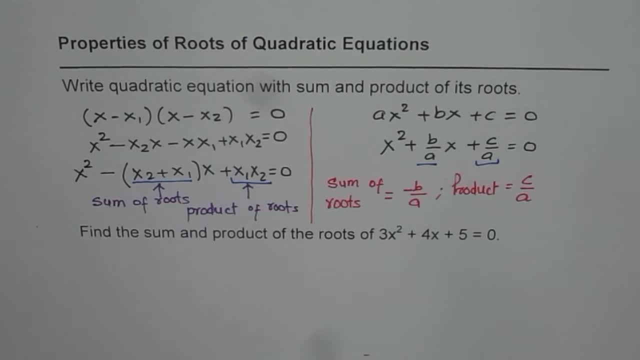 Do you see that Now, in these set of videos, we are going to explore this relation and find solution to many different variety of problems. Now, to start with, here is the first one. Find the sum and product of the roots of 3x squared plus 4x plus 5 equals to 0.. 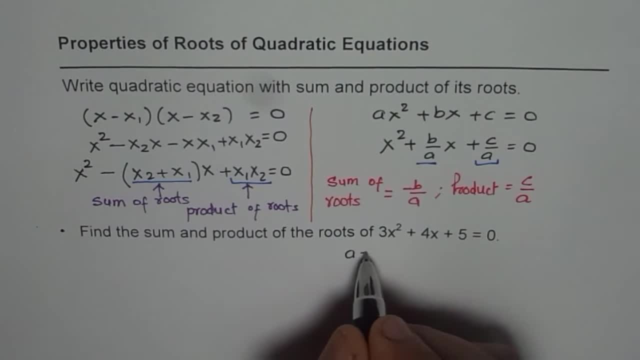 Now, in this equation, what is a? a is equals to 3x, b is equal to 3x, b is equal to 3x, b is equal to 4x, b is equal to 3x, b is equal to 4x. 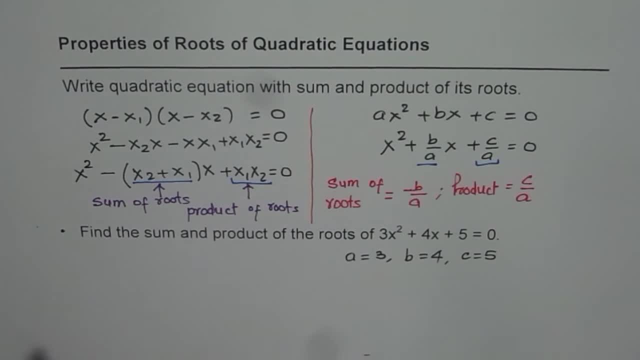 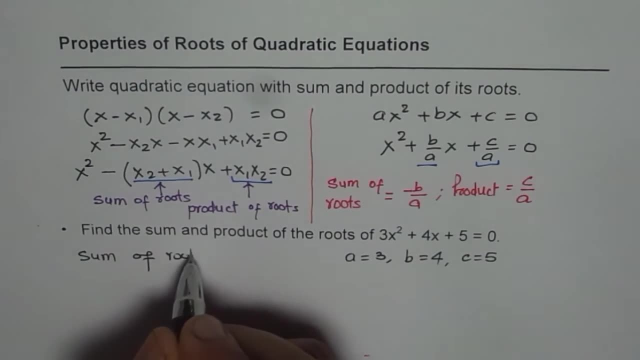 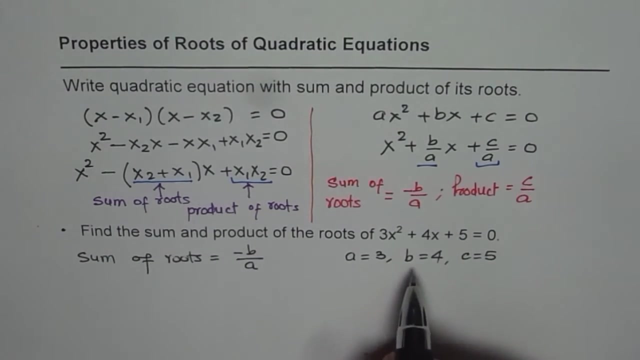 c is equal to 5x, c is equal to 5x. So from this, what we developed just now, what is sum of roots? We can write: sum of roots is equal to minus b over a, Minus b over a. 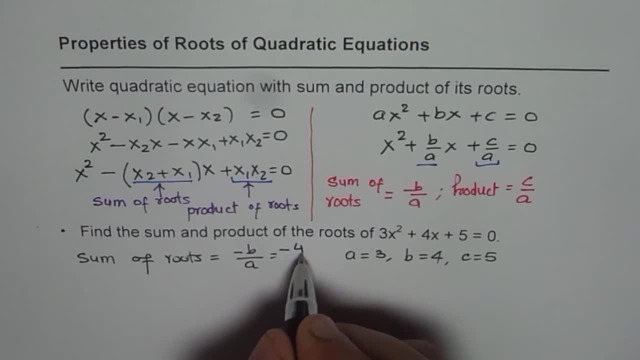 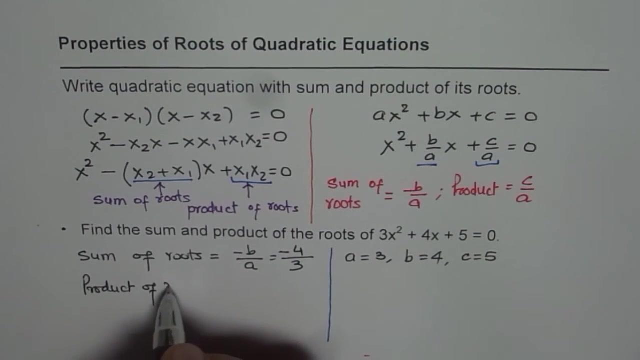 b is 4. And therefore it is minus. 4 over a is 3.. So that is sum of roots. And what is sum of roots, Correct? And what is product of roots? Product is c over a, c is 5.. 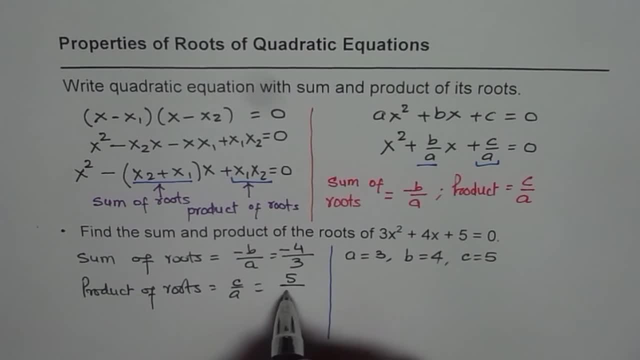 a is 3.. 5 over 3.. So that is how you can solve this. I hope you understand the concept and you also understand, if I give you the sum of roots, then what is going to be the quadratic equation. I mean 2.. 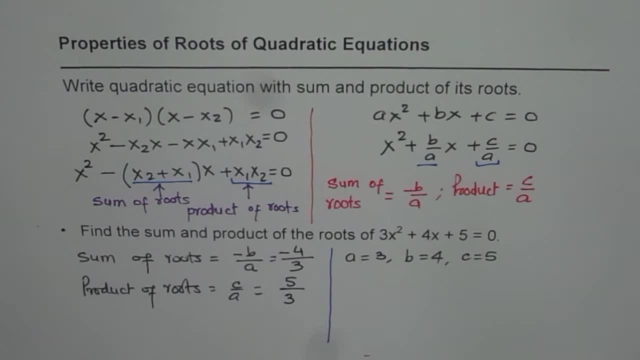 sum and product of roots, then what is going to be the quadratic equation? right? so this equation i could written write with the help of these two. also right, if i use these two, i can write the quadratic equation as: as what? let me write the x square minus sum of roots, which is minus 4 over 3. 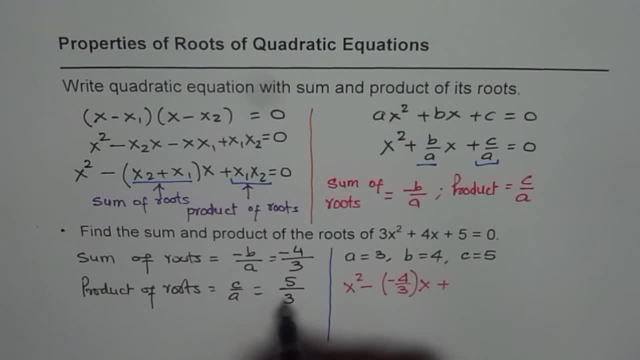 x plus product of root 5 over 3 equals to 0. now if i multiply everything by 3, what do i get? i get 3 x. square minus minus becomes plus 4 x, and here i get: plus 5 equals to 0. do you see that, so that? 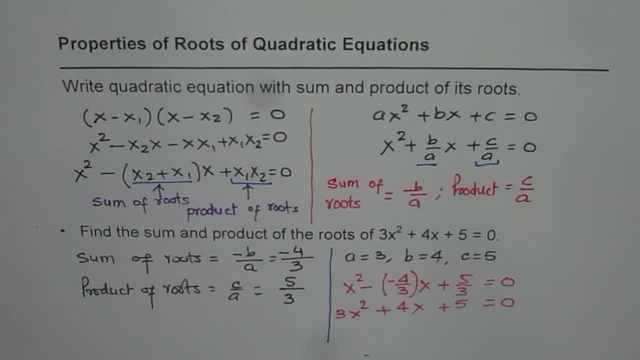 is how the roots are related with the equation. i hope that makes it absolutely clear. let's move on and do some interesting questions based on this learning. thank you and all the best. 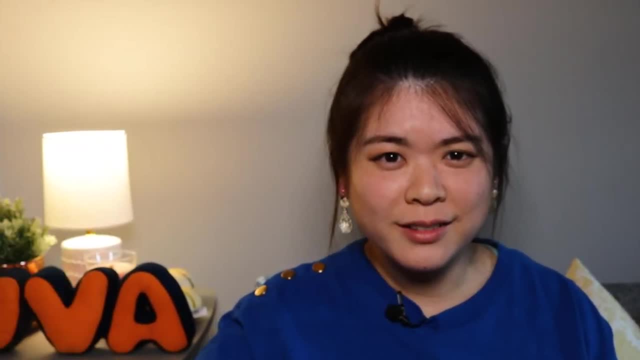 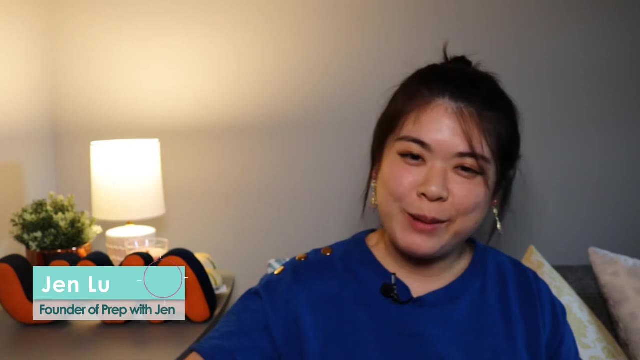 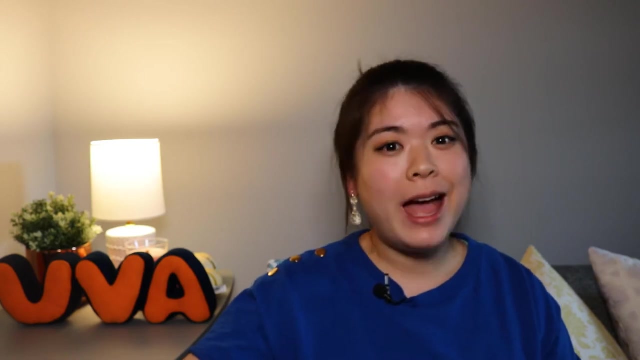 Constants Coefficients- What the heck are those? Hey guys, it's Jen. I'm a test prep tutor and today I want to share with you a couple of SAT math questions that have really funky wording If you have any amount of experience taking SAT exams. 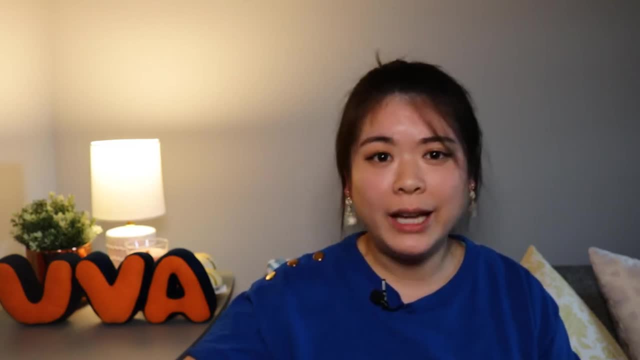 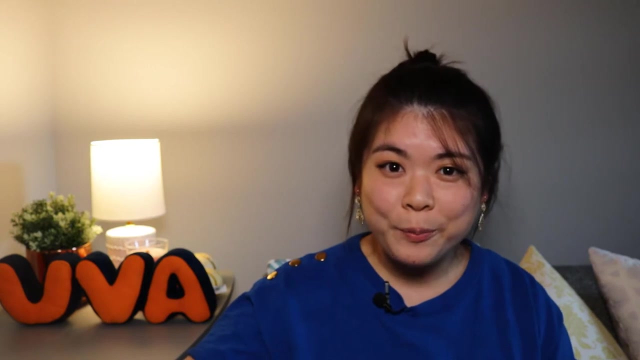 then you'll know that half of the battle is figuring out what the heck they want you to do. One of the trickiest types of questions are these quadratic equations that involve constants and coefficients. I know a lot of students struggle with these because they haven't seen anything like it in school. Now, this video was actually requested by somebody who 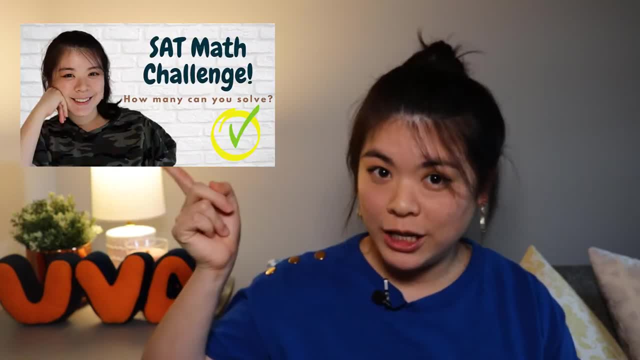 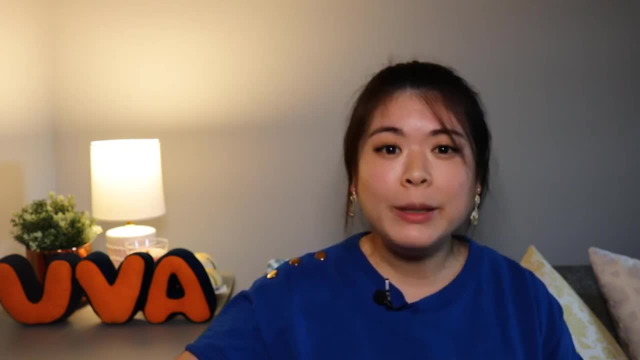 saw my SAT math challenge video. I'll link that up here if you haven't seen it. You should check that out. If you guys have any other questions you would like to see worked out, let me know in the comments. I do read those and they help me. figure out what to do with the questions. If you have any other questions you would like to see worked out, let me know in the comments. I do read those and they help me figure out what to do with the questions. If you guys have any other questions you would like to see worked out, let me.